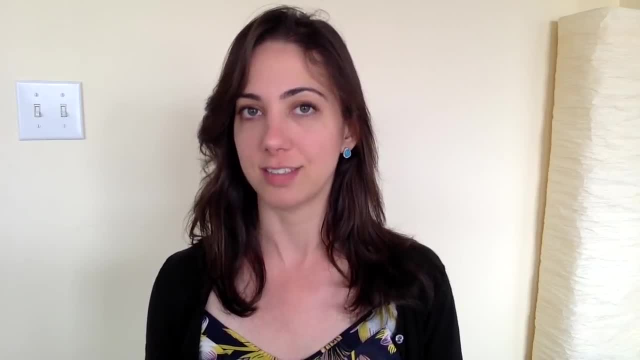 how can you tell the extroverted mathematician? And the answer is: he's the one looking at your shoes instead of his shoes, Anyway, so I think that observation is accurate, but there's another piece of information that's relevant and that people tend to forget when 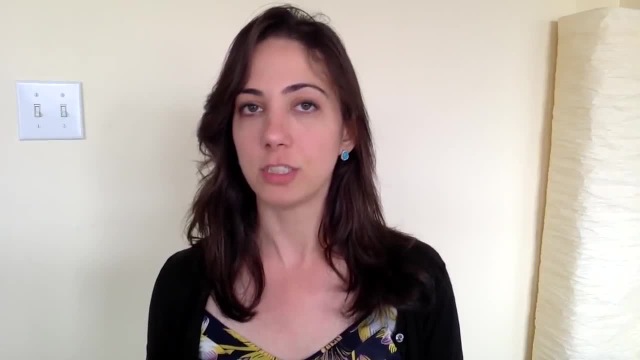 answering this question, and that is: how many math PhDs are there relative to business school students? There's a lot fewer. The numbers will vary from school to school, but it's something on the order of 10 times as many business school students as math PhD students. So 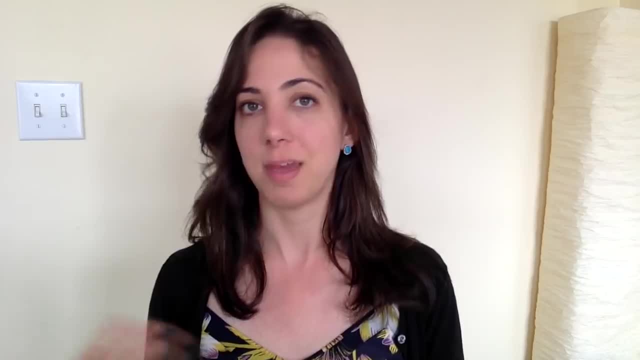 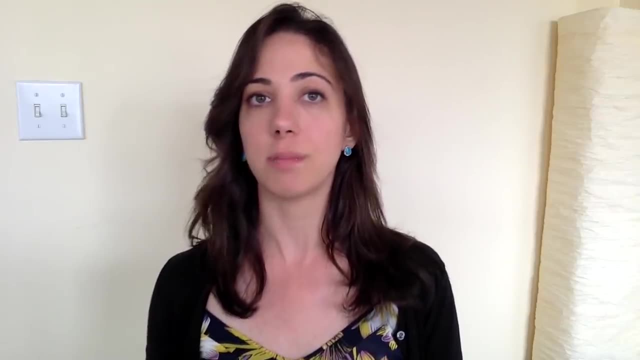 we have these two pieces of information about there being many more business students than math students and also about shyness being more common among math students than business students, And the question is: how do we combine these two pieces to get one overall estimate? 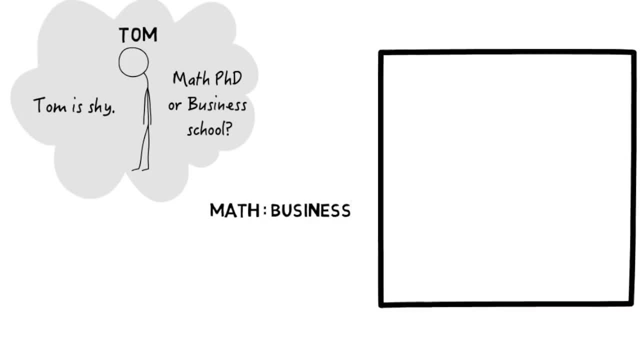 about Tom. This is where Bayes' Rule comes in, So you can imagine that this divides. you know the number of math PhD students and the number of business students that are in the class, So you can imagine that this divided rectangle represents the relative. 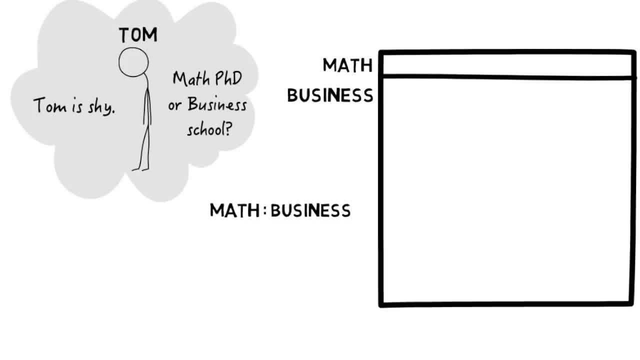 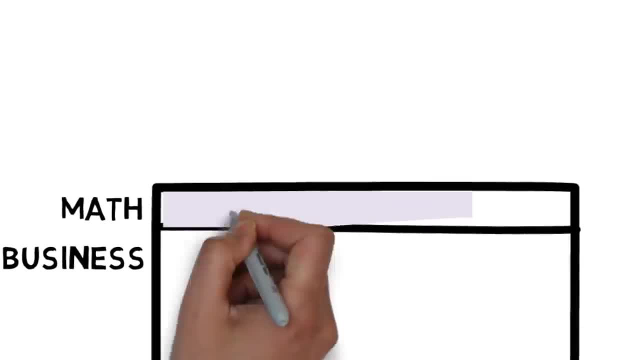 proportions of math to business students. very roughly speaking, We'll put it at one to 10.. And now, looking just at math students, we can ask: how common is shyness? I would very roughly guess that it's about 75% of math PhD students come off as shy. And now 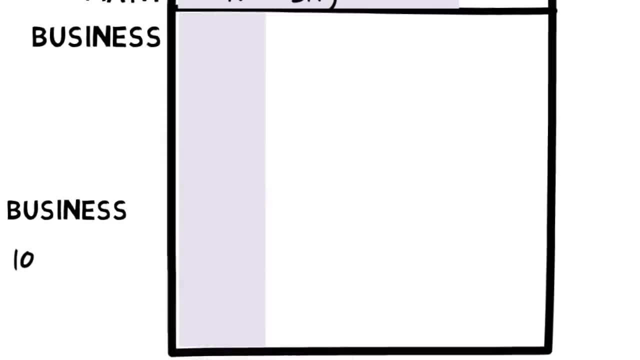 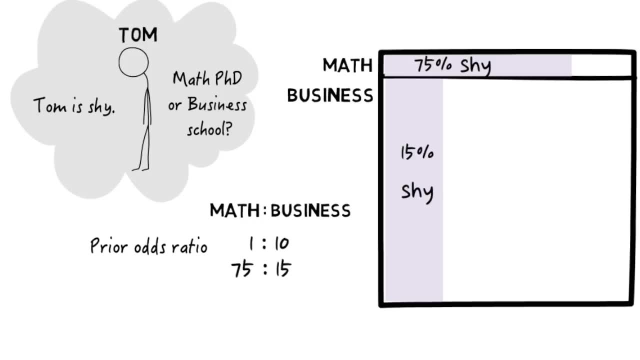 looking just at business school students- again guessing roughly, I'd say about 15% of business school students come off as shy. So now we've represented both of those pieces of information in one diagram and we want to know whether Tom is more likely to be in a math program or a business program. We don't. 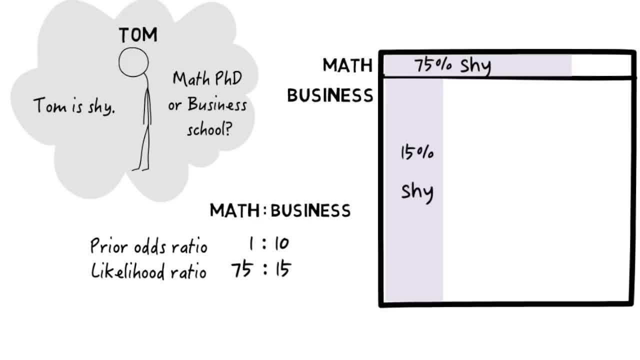 know which one he's in, but we do know that he's shy, which means that he must be in one of those lavender rectangles, right? Because those represent the shy math and the shy business students. So to get a sense of the relative probabilities of him being in math versus, 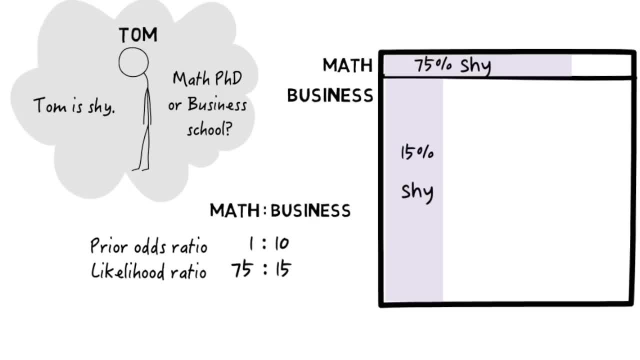 business. we just have to compare the relative sizes of those lavender rectangles. So we'll do that And it looks roughly like. the lavender business rectangle is about twice as big as the lavender math rectangle, And you can see how the math shakes out. We just multiply. 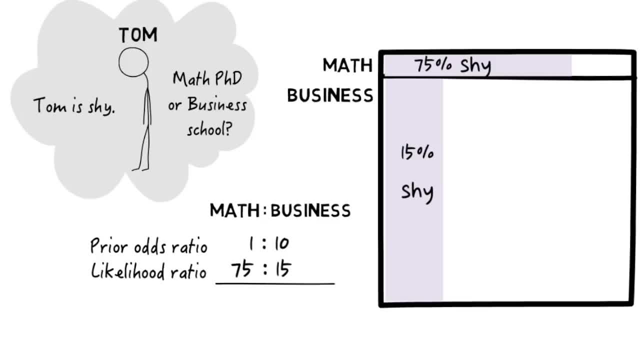 two linear ratios: the ratio of math to business students, which we put at one to 10, times the ratio of shyness in math versus shyness in business, which we put at 75 to 15.. And multiplying those two linear ratios gives us a ratio of areas which comes out to about: 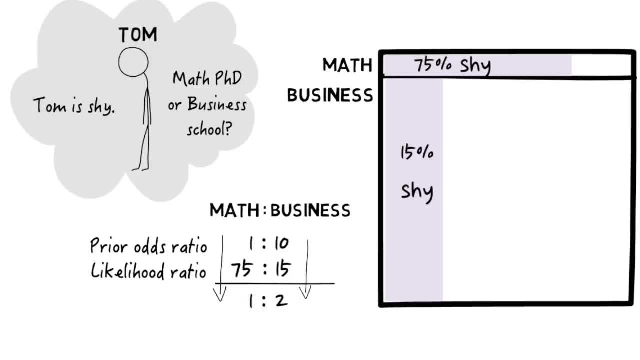 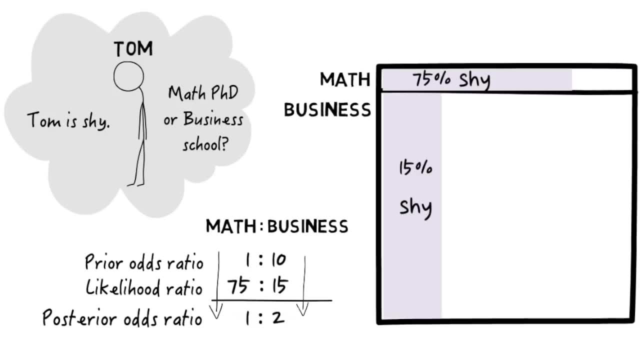 one to two, So roughly twice as likely for Tom to be in the business program. And then in the bracket of jogo ra, we can substitute a new line to the ball Korean, even though shyness is more common among math students. 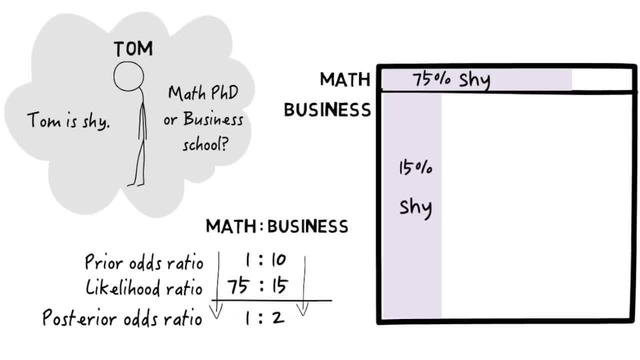 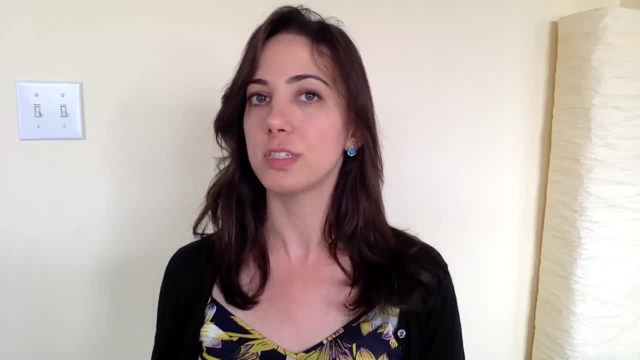 So this is the mechanics of Bayes' rule. This is how it works, And now I want to talk about how I use it in my everyday thinking. I don't plug numbers into a formula- I almost never draw these diagrams, in fact- But there are a few rules, principles of thinking that 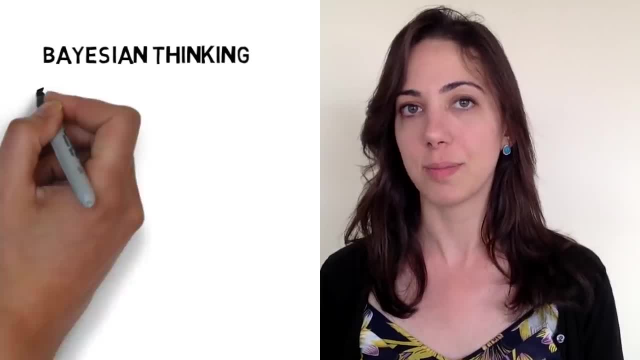 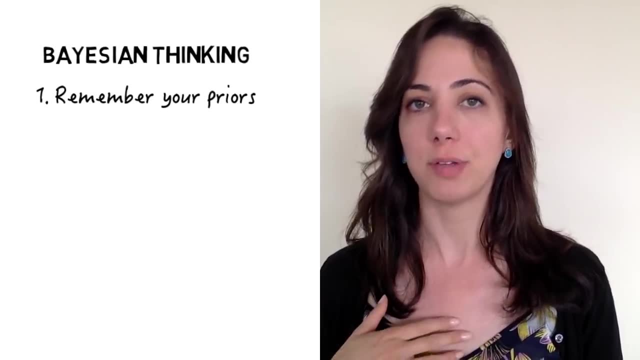 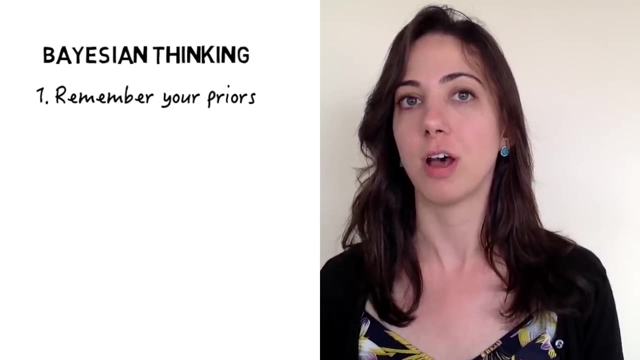 fall out of the math of Bayes' rule that are really useful for me. So, as you saw in the Tom example, what people naturally do is focus on the evidence that Tom is shy and forget about the prior, the sort of background knowledge that math is. 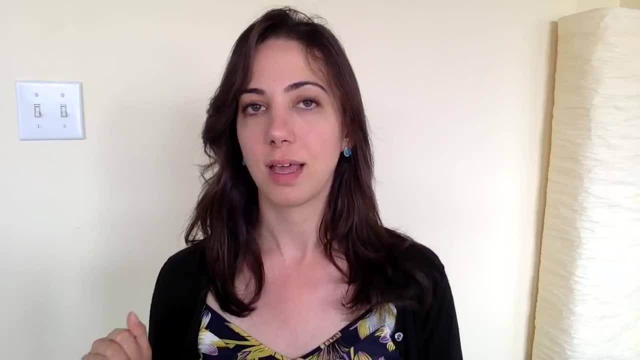 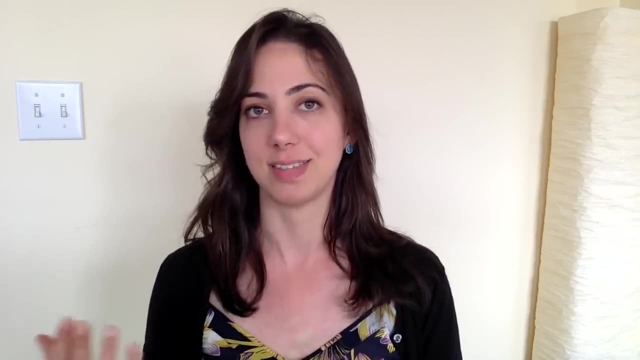 just a much less common major or program than business. And this is a very common phenomenon. it's called base rate neglect And a personal example. I have many examples of this myself, but one example comes recently from: I rented a house with some friends and while we were there we had to call a repairman. 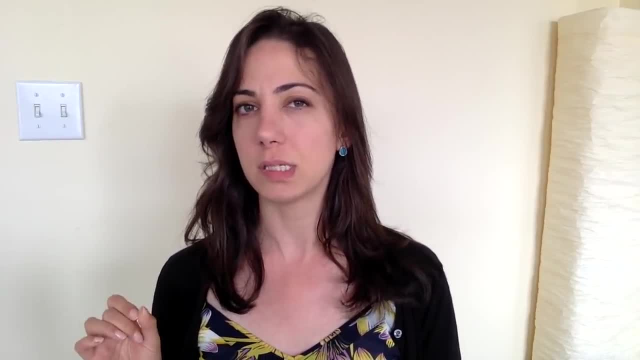 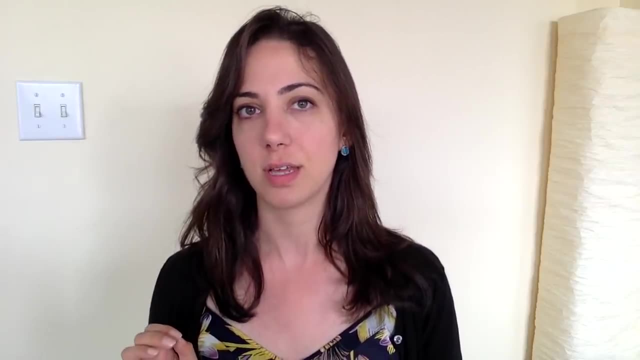 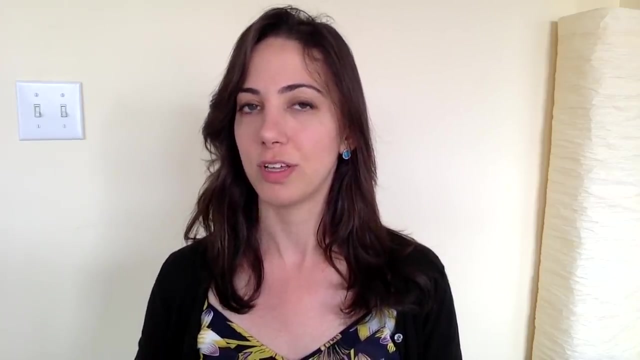 to fix the stove And he made us a little bit nervous because while he was there we noticed him sort of peering into different rooms of the house and there's no reason you would need to see the bedroom of a house if you're here to fix the stove. 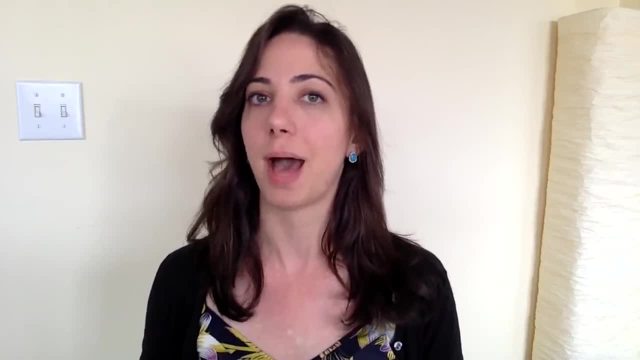 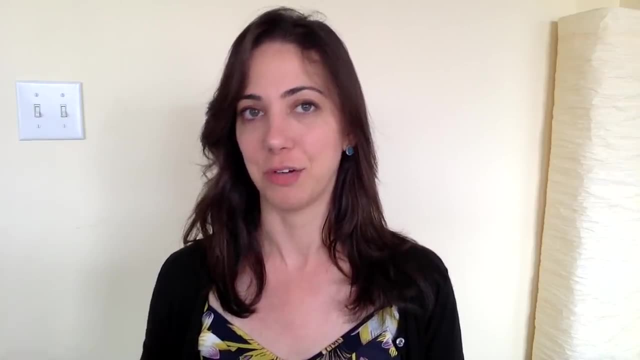 So we had heard stories in which repairmen come back after having done their repairs And rob a house after having had a chance to you know, case the joint or whatever, And so we were worried that that was what was going on in this case. 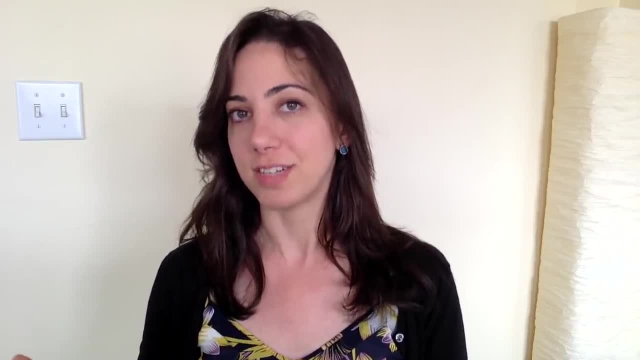 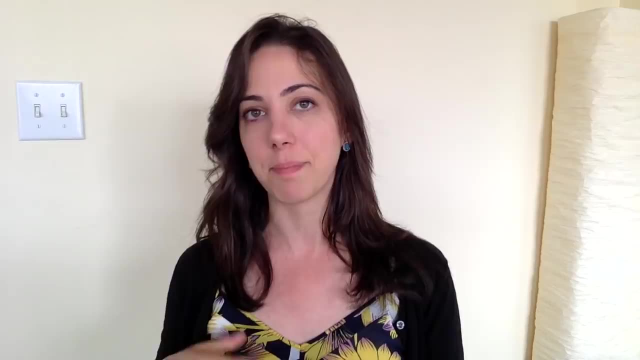 And I think that seeing your repairman snooping is some evidence that should make you somewhat more confident that he's going to rob you. But we had to take a step back and remember what is the prior on a repairman being honest versus a robber. 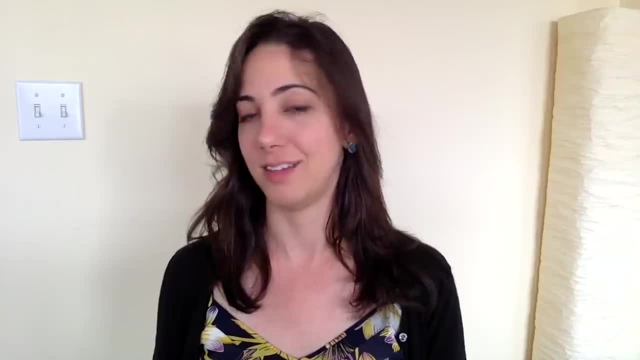 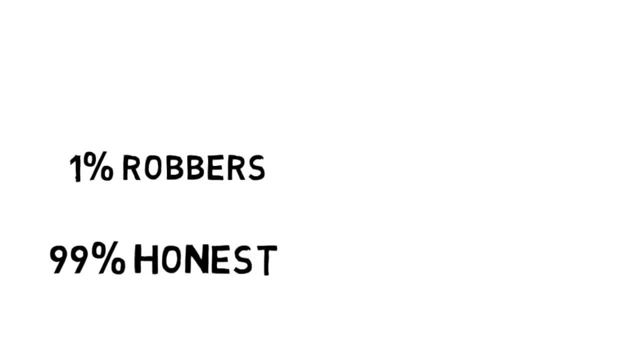 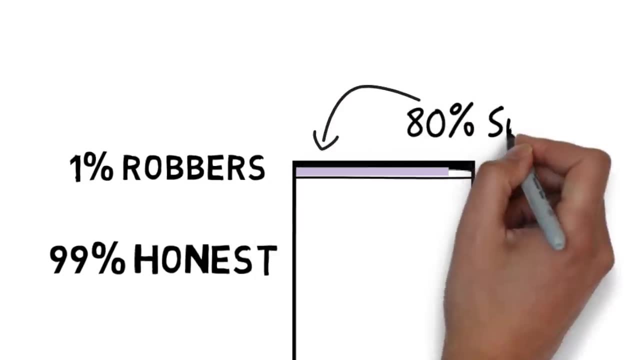 than robbers, Something on that order. So even imagining that snooping is much more common among robbers than honest repairmen, let's say 80 percent of robbers will be seen to be snooping, and maybe 10 percent of honest repairmen. 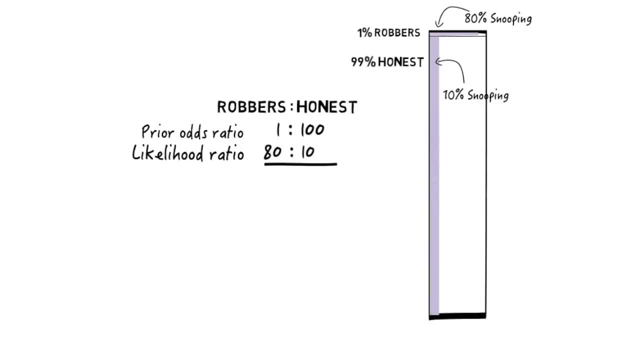 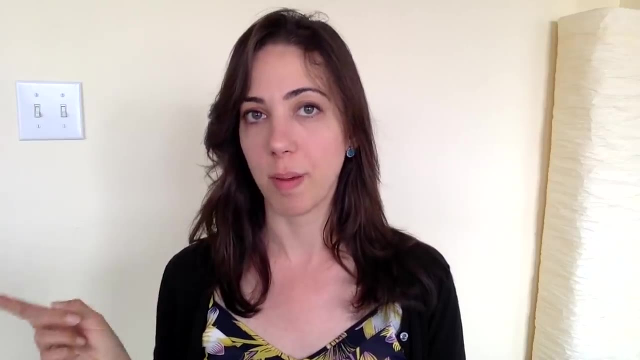 Even so, seeing that evidence should only bump our probability of this guy wanting to be a robber- maybe 8%. So you know we should lock our doors but not freak out Something like that. So that's principle number one. remember your priors. Principle number two, I'll illustrate. 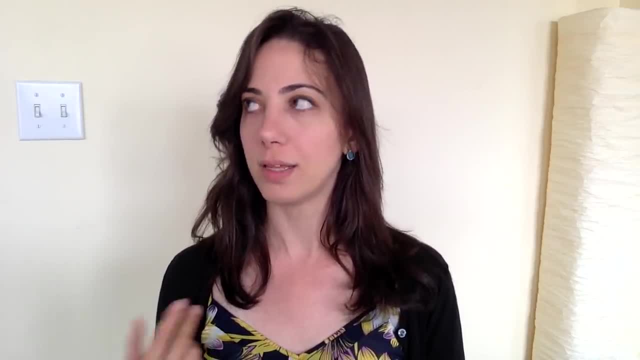 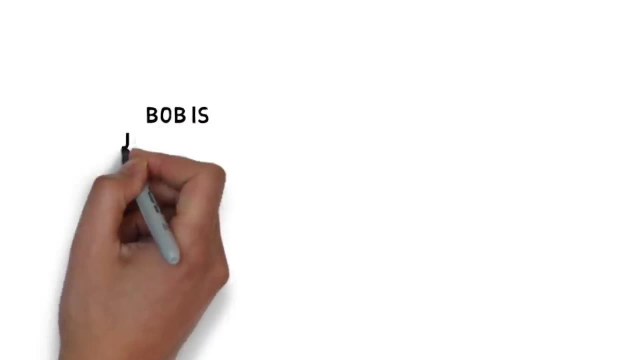 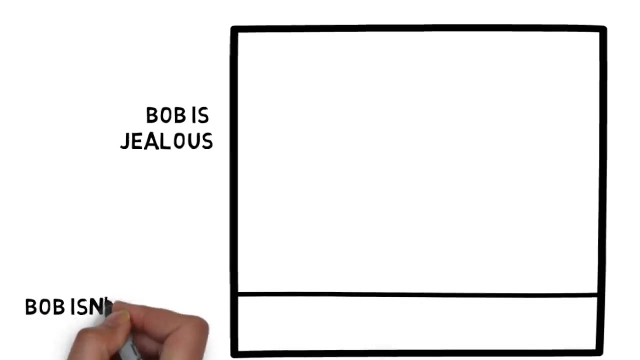 with another story from my life. A while ago I was working with a guy named- let's call him Bob- and I had reason to believe that Bob might be jealous of, or competitive with, another person who worked with us- Let's call her Alice. So one day I'm having coffee with Bob and he's 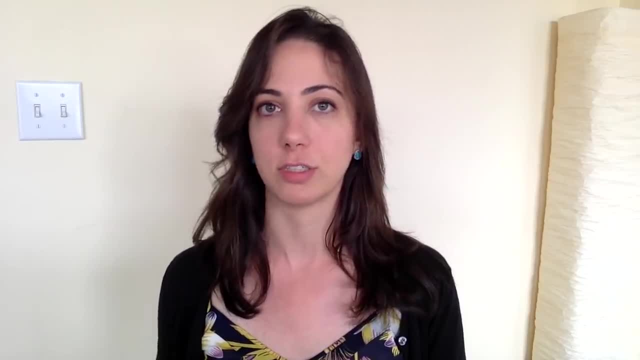 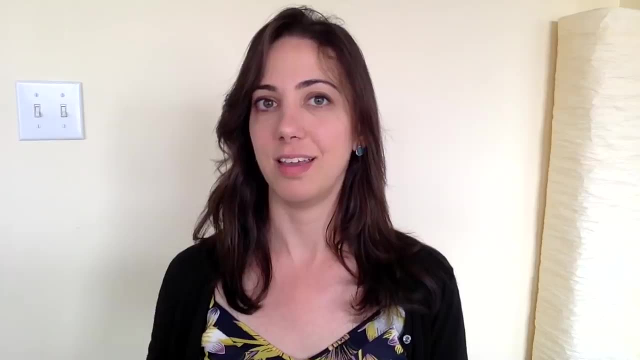 complaining about Alice, I think, because she hadn't finished some project that she was supposed to have finished by that point. And I'm thinking to myself, this just proves that I was right about Bob. If he was jealous of her, he would want to make her look bad, and he's complaining about her. 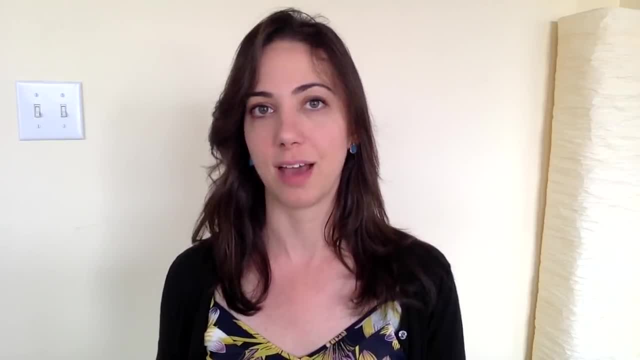 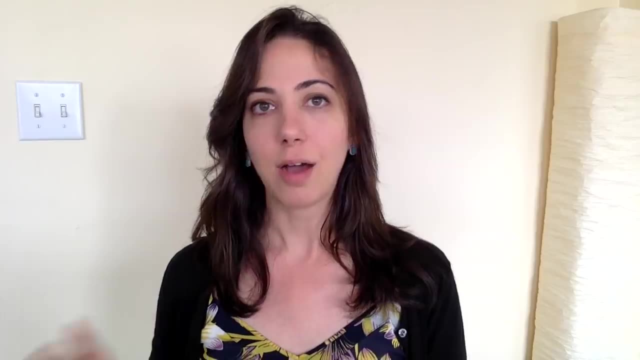 so I'm right. And a little while later it occurred to me to ask: well, okay, let's assume for the moment that I'm wrong and Bob is not jealous, Alice, How implausible is it really in that scenario that he would be complaining about her? 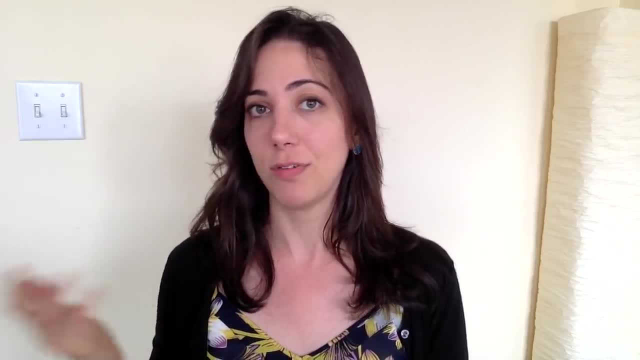 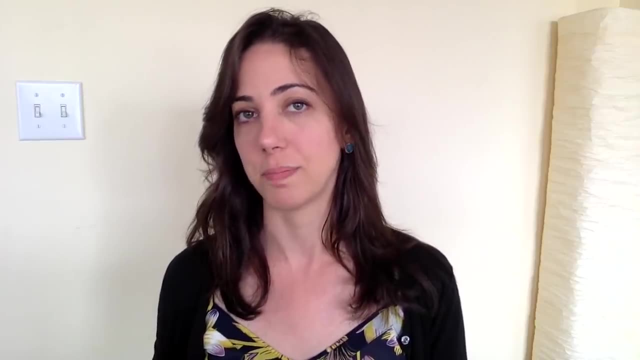 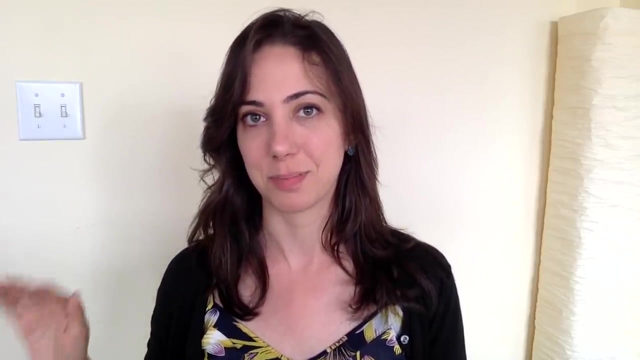 And it's not implausible at all. actually, It often happens that people get annoyed when someone doesn't finish something that they were supposed to finish, and it doesn't have anything to do with being jealous or competitive, And so I may still have my prior reasons to suspect that. 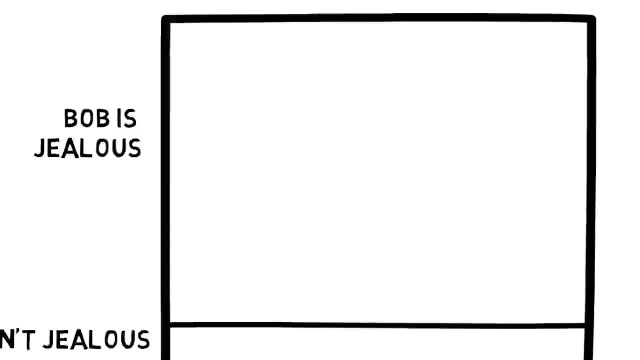 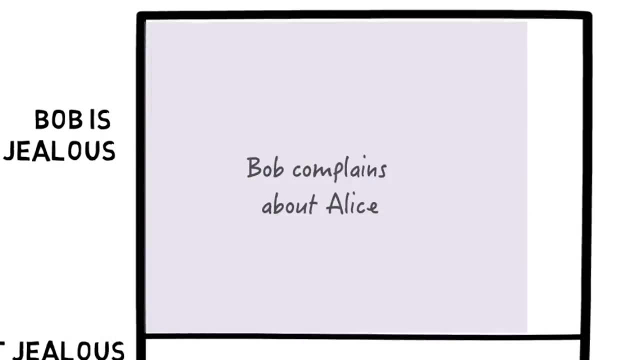 Bob is probably jealous of or competitive with Alice, but seeing this new piece of evidence should not make me feel significantly more confident that I'm right. Maybe complaining about Alice is a little bit more likely in the world in which he's jealous of her than in the 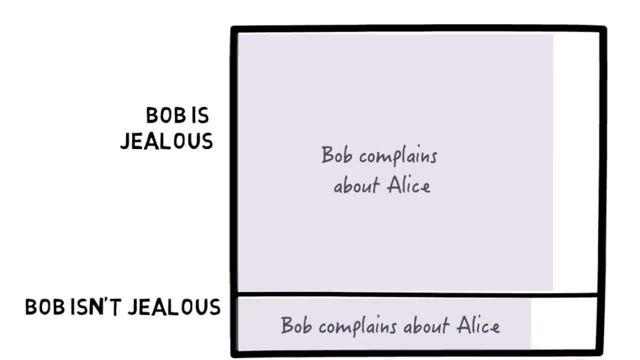 world in which he's not, but only slightly. It should not really shift my probability that much at all that I was right, And I think that this is a very common thing as well, that we go around the world seeing pieces of evidence that we can explain with our current theory, with our pet. 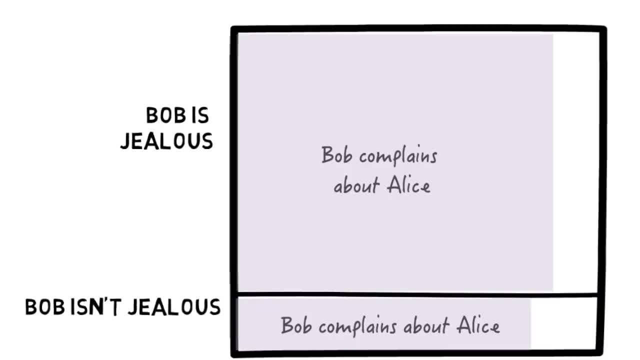 theory, and that makes us feel all the more confident that we're right And we don't take that extra step of asking: well, what if I were wrong? What would I expect to see then, And how different is it, if at all, from what I see now? So I keep this principle in. 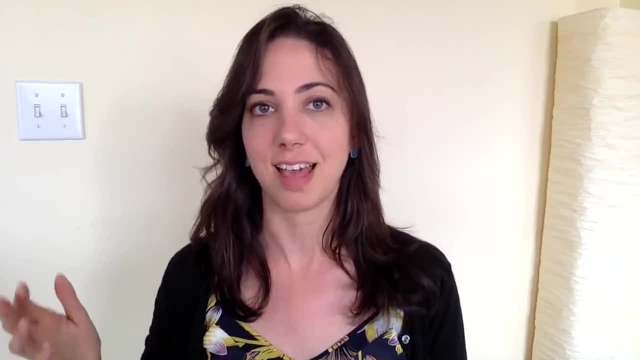 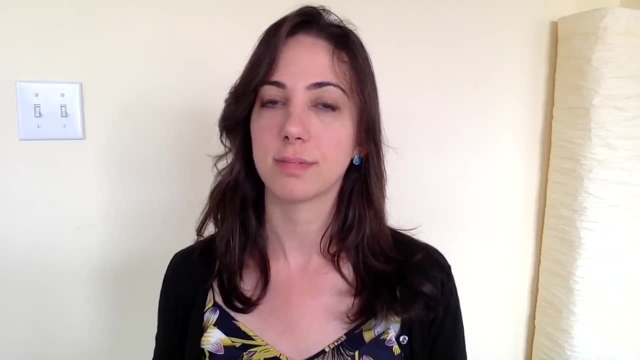 mind when, let's say, I try some new diet and I notice that I have more energy this week. Well, how likely is that in the world in which the diet doesn't work compared to the world in which it does? Maybe my energy is really very variable, so it's not really that implausible that my energy 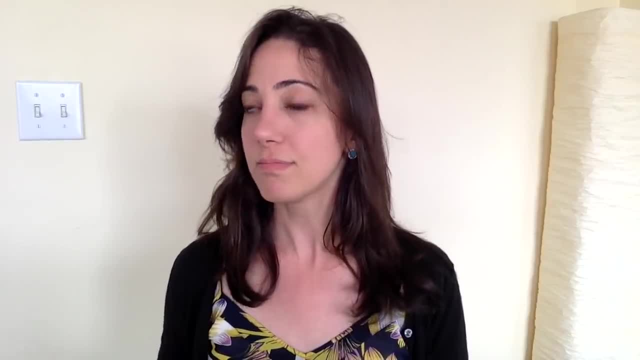 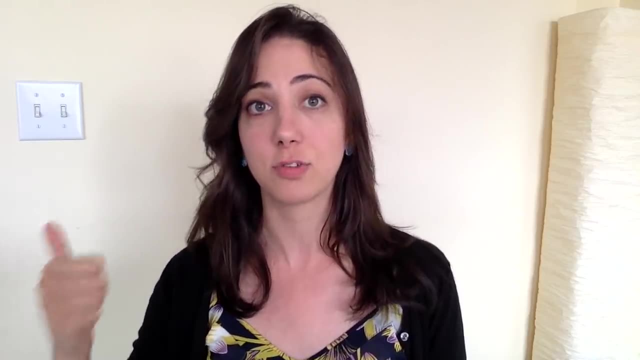 would happen to be higher right after trying to eat something. So I keep this principle in mind when I'm following the diet. Or let's say, I give someone a paper or an idea to evaluate and he thinks it's great. I have to ask myself: well, how common is it for him to think that bad ideas are? 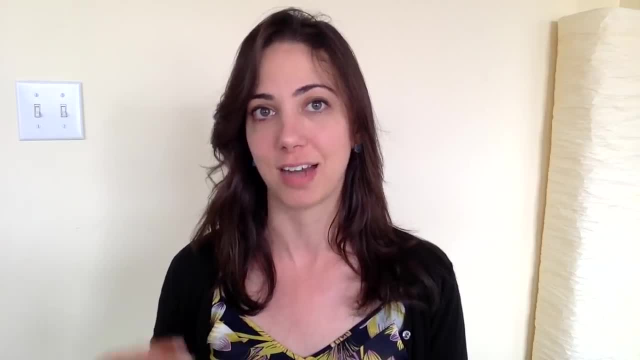 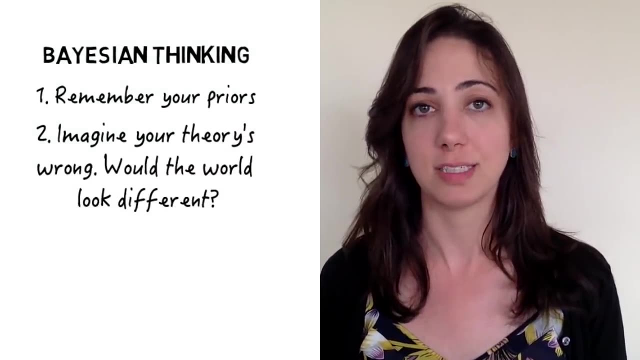 great. How much evidence is his approval that my idea is in fact great? So that's principle number two. Ask yourself what if I were wrong? What would I expect to see, And how is it different from what I currently see? Principle number three is sort of the flip side of principle number two. 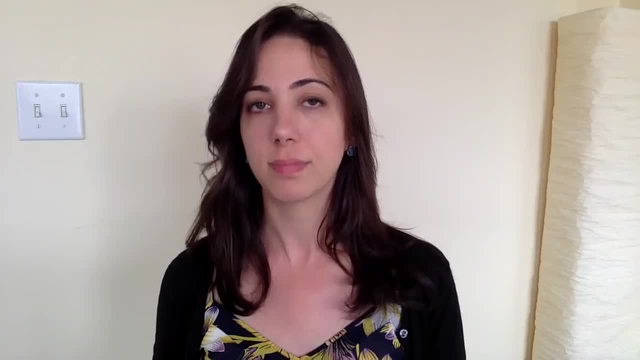 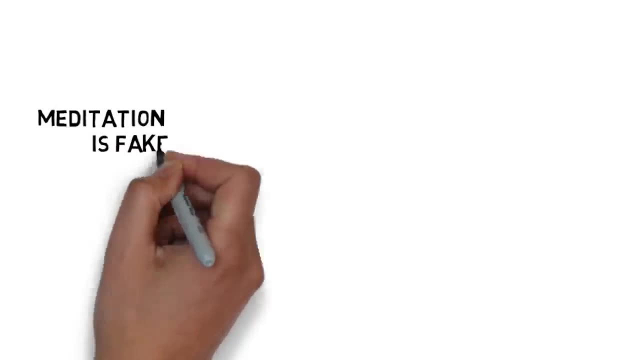 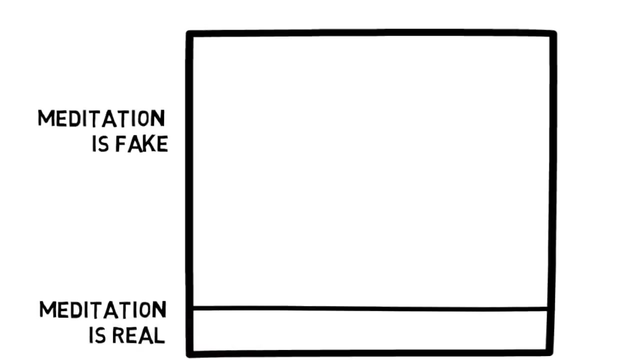 You could call it update incrementally. So another story: When I first moved to Berkeley, I was pretty confident that meditation was- for lack of a better word- fake, And so I was surprised when one of my friends that I met in Berkeley, who was very smart and thoughtful, 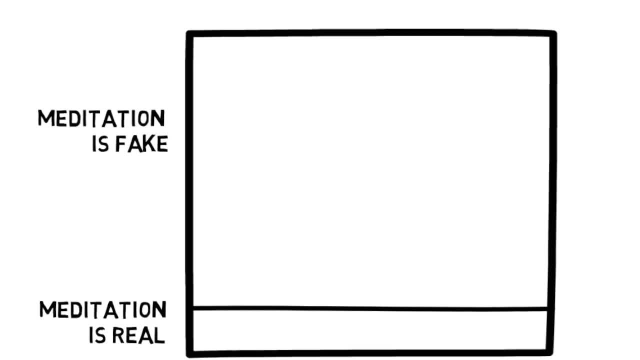 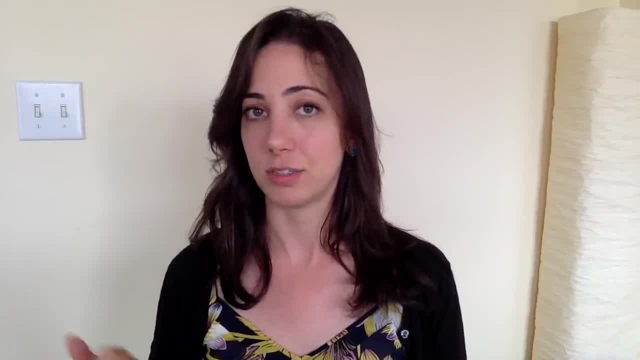 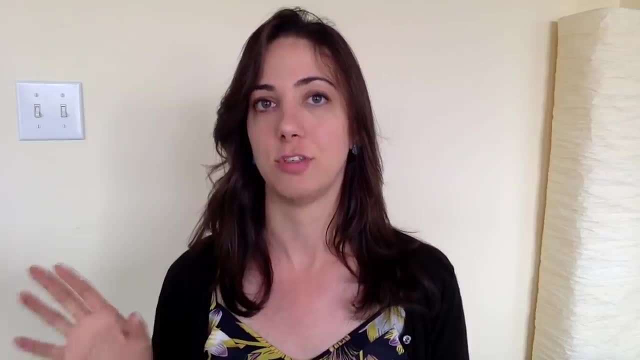 he raved about meditation and said it had made him much happier as a person, And I think it's very easy to explain this evidence away by saying: well, there's a placebo effect there. He expected meditation to work and so he felt that it did, Or maybe there was something else in his life that 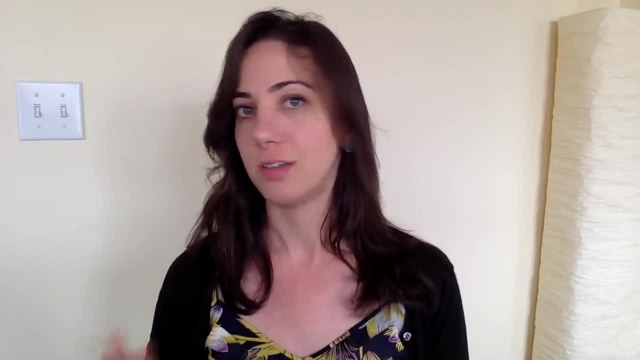 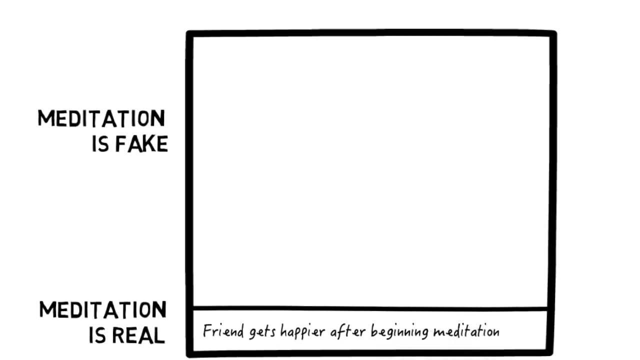 changed around the time he started meditating and that was actually making him happier, not the meditation, And I think both of these stories are totally plausible, But I have to admit that it seems at least a little bit more likely that my smart, thoughtful